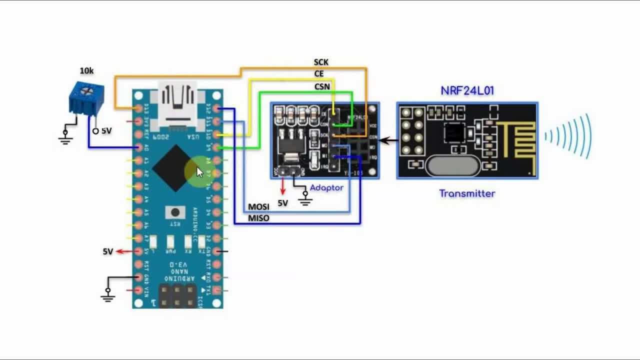 the clock is connected to pin D13, the master-out slave input is connected to pin D11, and the master-in-slave output is connected to pin D12.. We also have a 10K pot connected to analog line A0 of the Arduino. 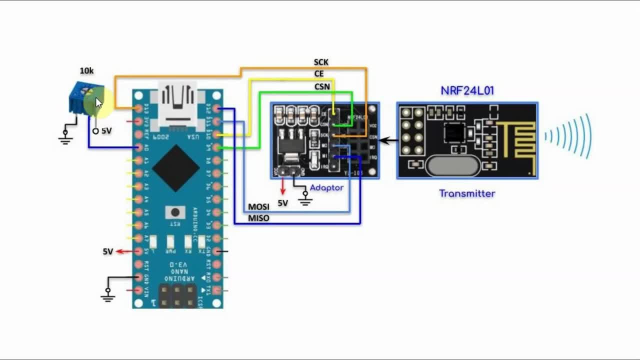 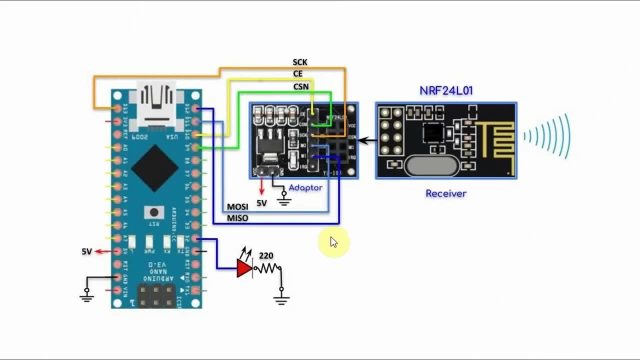 The pot will be used to control the blinking speed of an LED connected at the receiver side. This is the receiver circuit, which is similar to the transmitter one. We have an LED here connected to pin D2 of the Arduino. The LED will blink based on control signals coming from the transmitter. 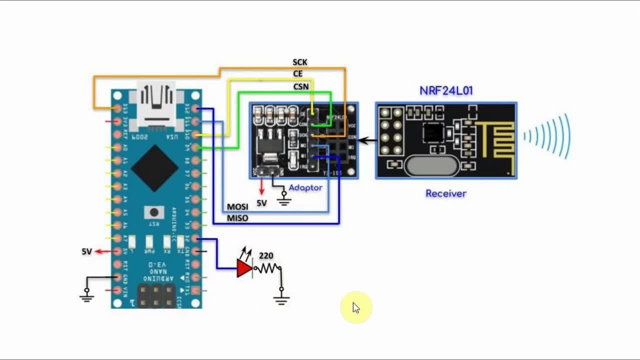 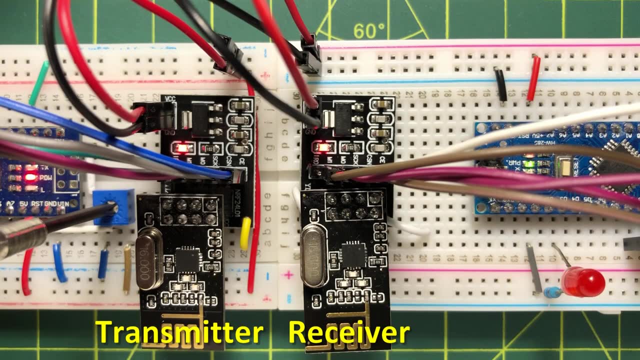 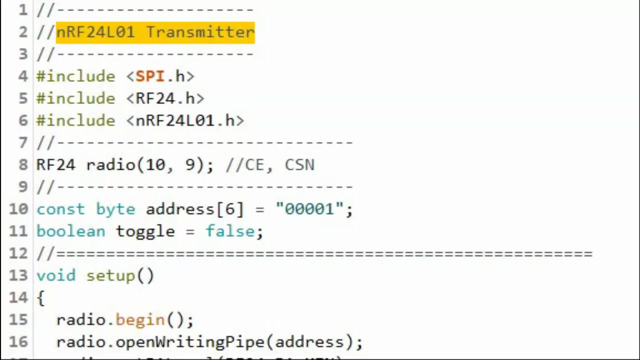 In the pot connected at the transmitter will be used to control the blinking speed of the LED. And now for a quick demonstration. If let's have a quick look at the transmitter sketch. we need to include the SPI library so that we enable the SPI protocol, and we need to include 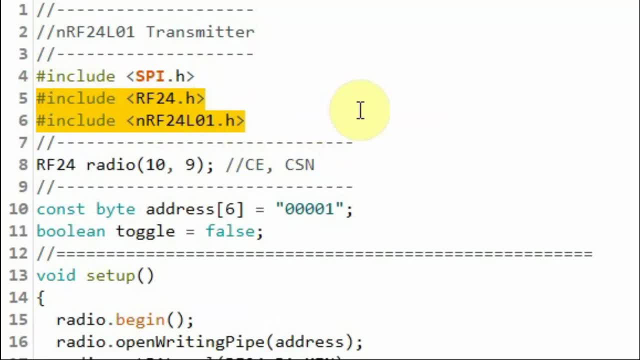 these two libraries so that we can access the nrf24l01 module. we need to create this object radio and we need to indicate where the chip enable pin is connected on the Arduino and the chip select, not pin. next we create this byte string called address, which will contain the address of the receiver and the 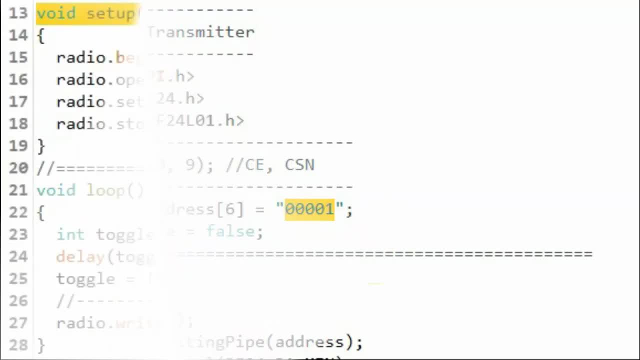 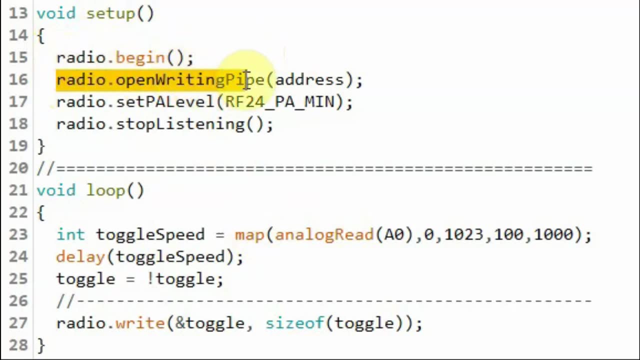 address is a five character string. inside this SETTF function we initialize the RF module and then we open a data pipe between the transmitter and receiver by providing the address of the transmitter and receiver, and then we open the transmitter and receiver by providing the address of the. 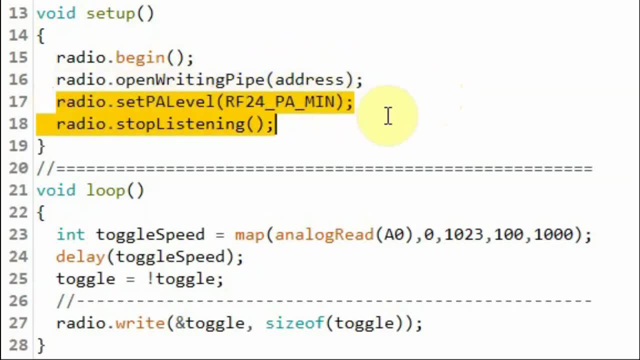 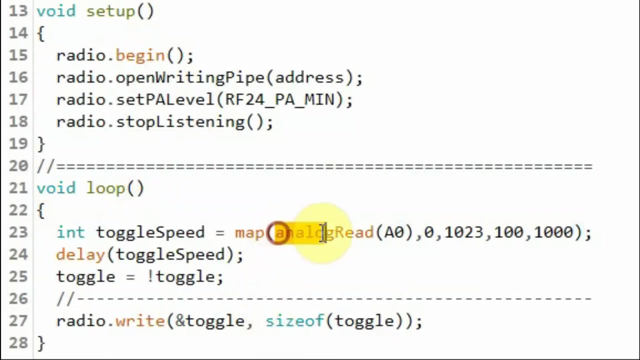 receiver and using this function here we are setting the power amplification of the transmitter to the minimum, since the two modules are in proximity. and in this function here- stop listening- we are establishing that the module here is a transmitter, not a receiver. inside the loop function we get the pot value and 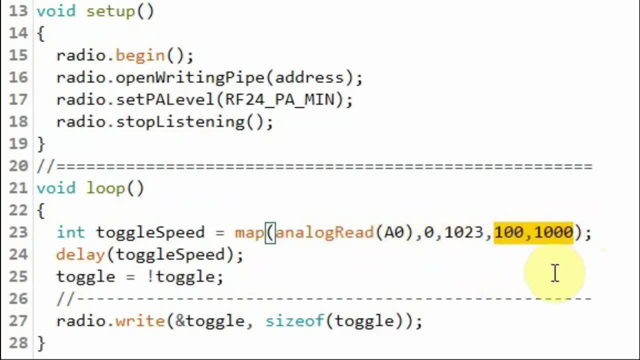 then we remap the value to a range between 100 and 1000 and then store this in this variable here, and then we use this variable as the argument of the delay function and then we negate the boolean variable toggle and then, using this function here, we send that variable, which could be either true or false, to 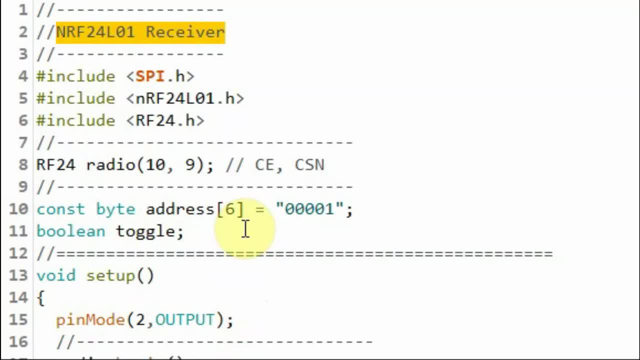 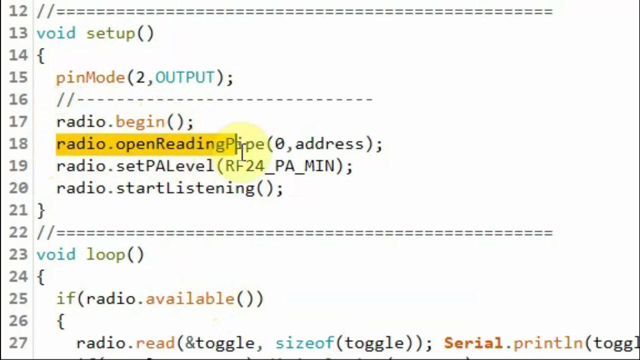 the receiver- and this is the sketch. at the receiver side, we include the same library as the transmitter one and we create the same object and we create the same address string, which will have the same address defined in the transmitter. inside the set of function, we initialize the RF module. we establish a data pipe. 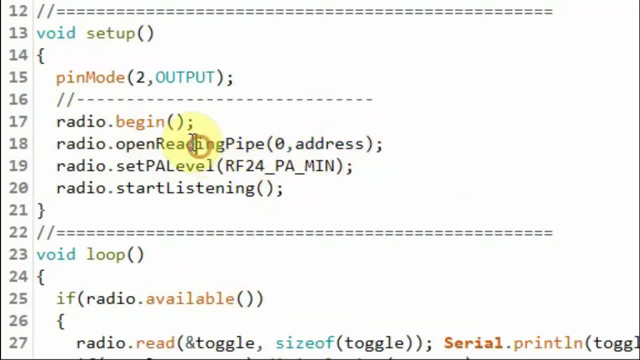 between the transmitter and the receiver. but here we using function open reading pipe, and this argument here represents the pipe network number. we could have up to six pipes, so from zero to five, and here this is the address of the pipe between the transmitter and the receiver. we set the 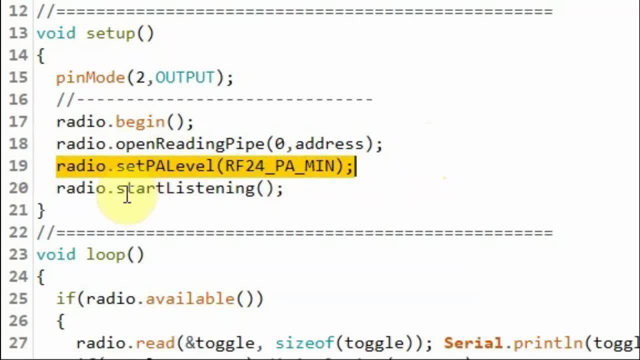 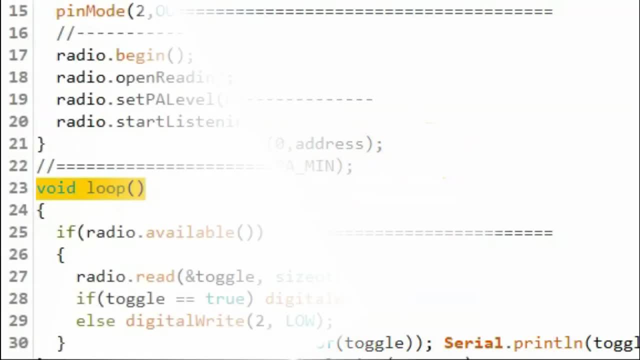 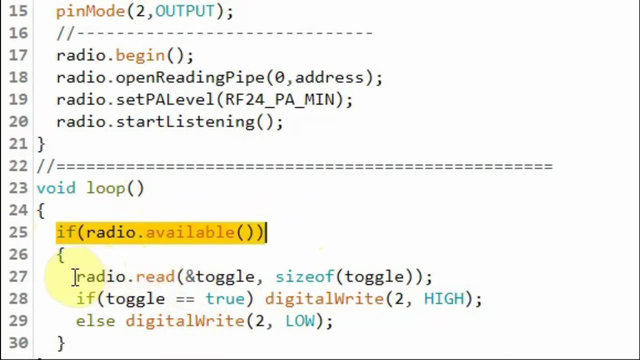 power amplification of the module to the minimum and then we set the module to start listening and meaning that it is now a receiver. within the loop function, we check whether we have data coming from the transmitter. if so, then we read the data and we store the data and this boolean variable toggle. 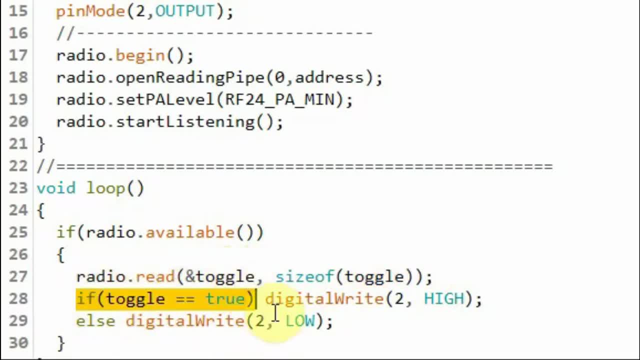 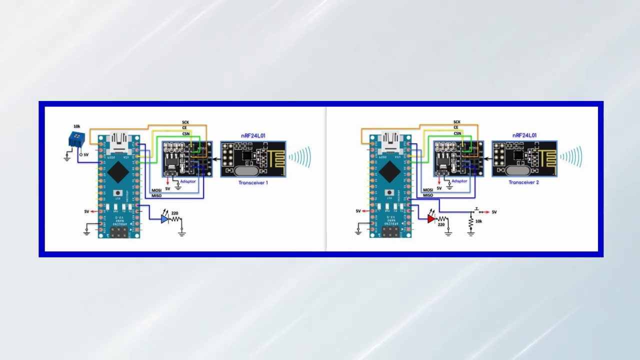 and then we check the value of toggle. if the value is true, then we turn on the LED. otherwise, if the value is false, we turn off the LED and the process is repeated and we have a blinking LED. the codes at the transmitter and at the receiver side have been modified, so now we have here to take the LE shape of the cable. so this is going to be a receivedonces here and to go on the Negotiator profile, we accept the data and the data is pressed in. we perform a several course results for the test to work. it looks like something is not much going to happen, but 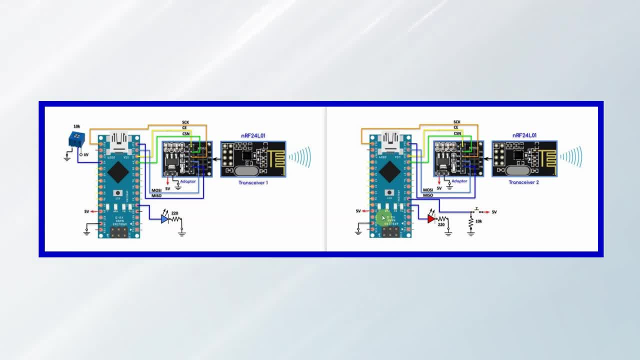 transceiver one and here we have transceiver two, which means that each system is capable of transmitting and receiving data at the same time. At the transceiver one side we have this 10k potentiometer is now is used to control the blinking speed of this LED at the transceiver. 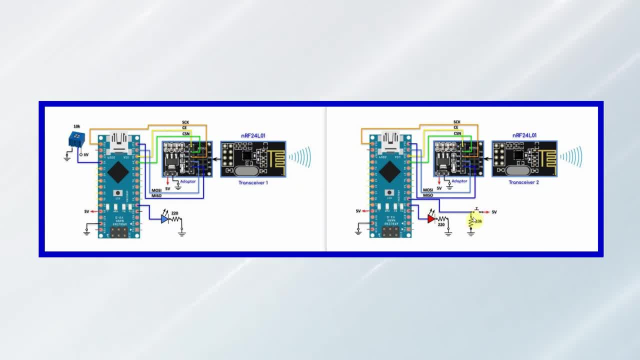 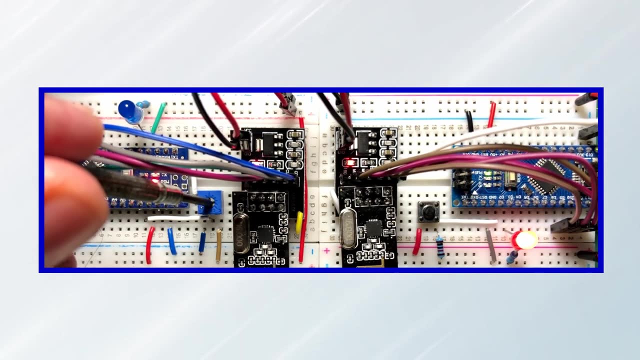 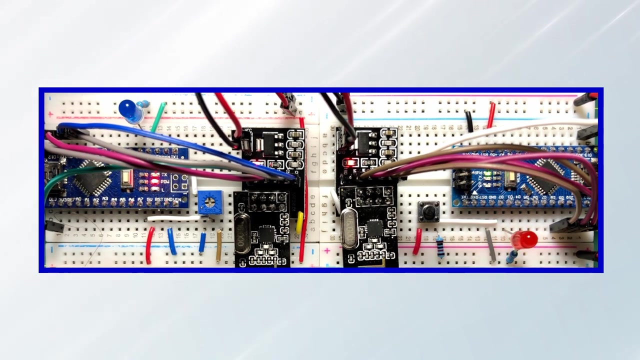 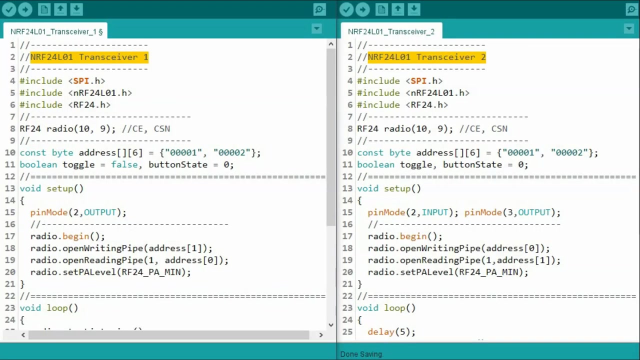 two side and we have here a push button at the transceiver two side is used to control the on and off of this LED at the transceiver one side. and now for a quick demonstration, a quick look at the sketches for both transceiver one and transceiver two. we need to define two. 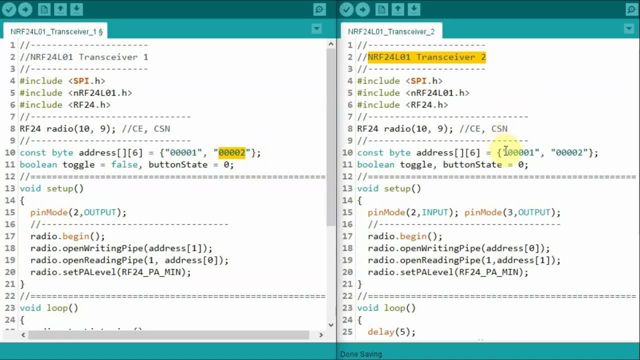 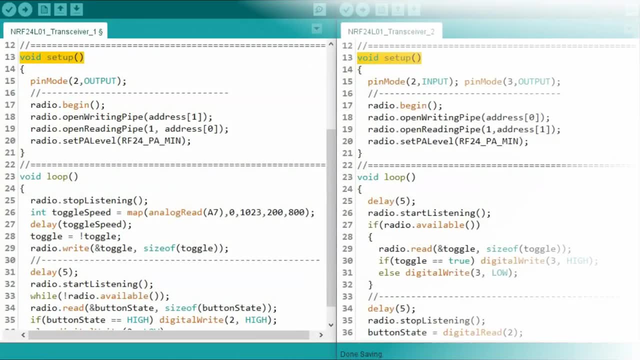 addresses or two pipes for each transceiver, since each transceiver will be transmitting and receiving data at the same time. Within the setup function of transceiver one, we need to initialize the function openWritingPipe and the destination address is address one, which is the address of transceiver two and at the other end of transceiver two side, 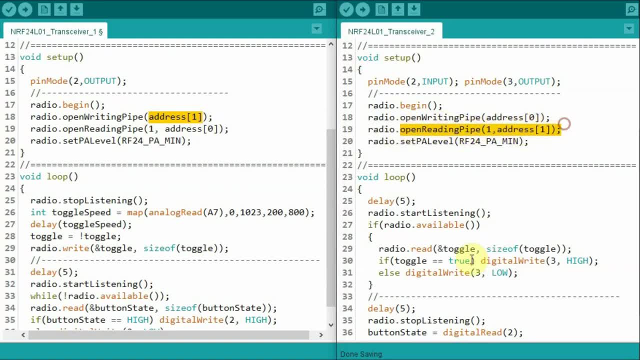 we need to open ReadingPipe to this address. Likewise, at transceiver to side, we need to open writing pipe to a destination address, zero, which is the address of transceiver one, And at transceiver 1 side we will have open reading pipe to this address. 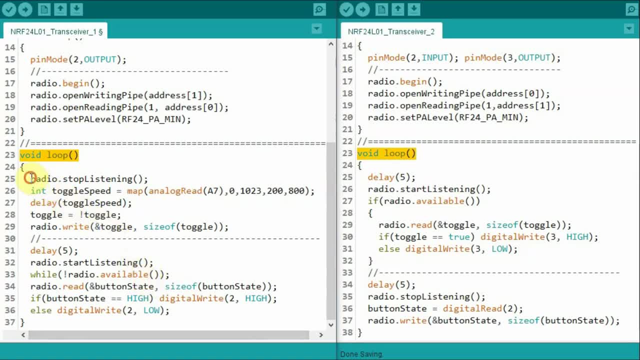 Inside the loop function of transceiver 1, this part of the code represents the transmitter part, while this part of the code represents the receiver part. When the transceiver 1 is a transmitter, it will take the boolean value of toggle, which is controlled by the 10K potentiometer. 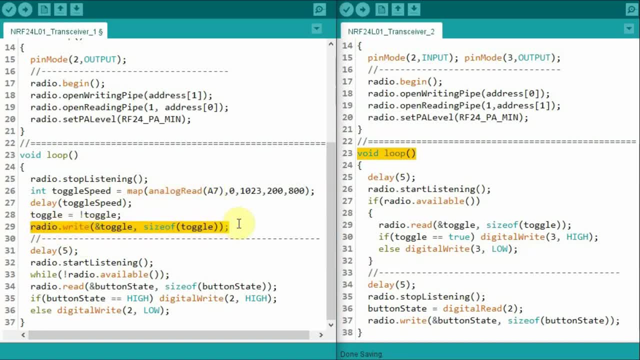 and it will send it to the transceiver 2 to control the blinking of the LED. When transceiver 1 is a receiver, it will wait for the status of the push button connected at transceiver 2, which is either on or off- and use it to control the LED connected at transceiver 1..